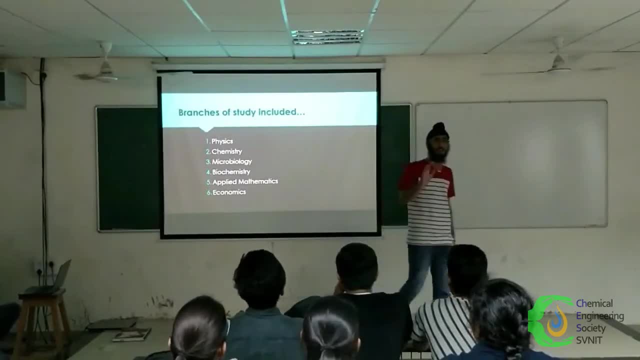 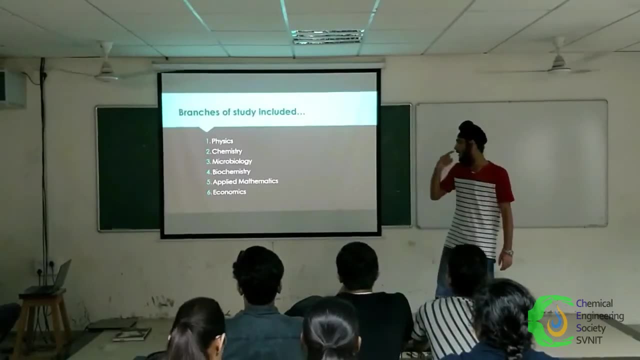 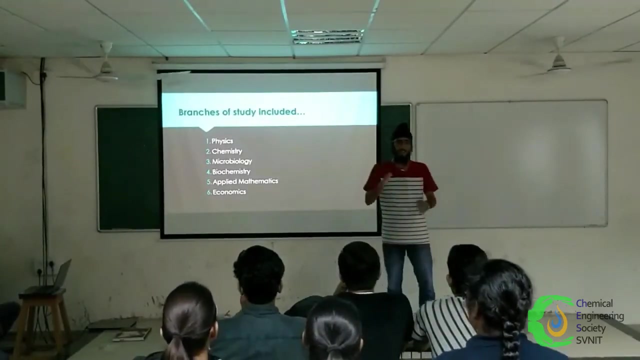 bhi bohat aati hai, and physics is the most important subject that you are going to study. in chemical engineering, Almost all the subjects involve physics. Chemistry is required only in three subjects and two of the subjects are chemical reaction engineering. So if 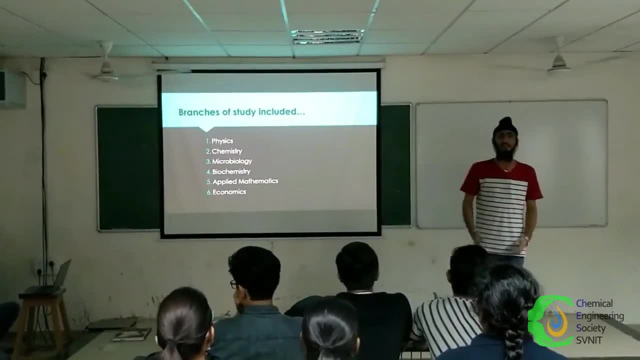 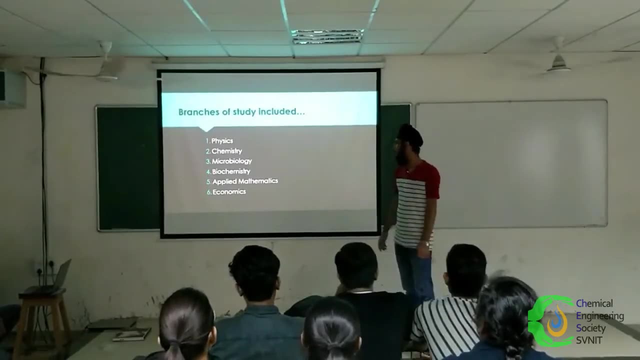 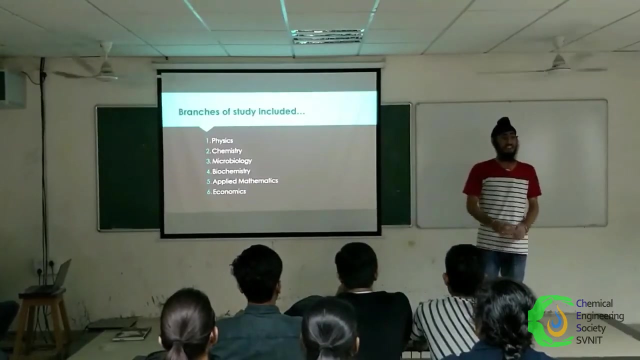 you are. if you thought that I am good in chemistry so I should take chemical engineering, I think that was. that is a myth that we all need to like break down right? So, and you see, ki, all these subjects- these are so many subjects, not all are taught in every other. 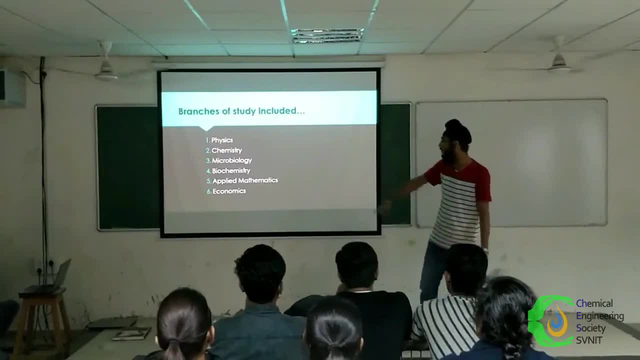 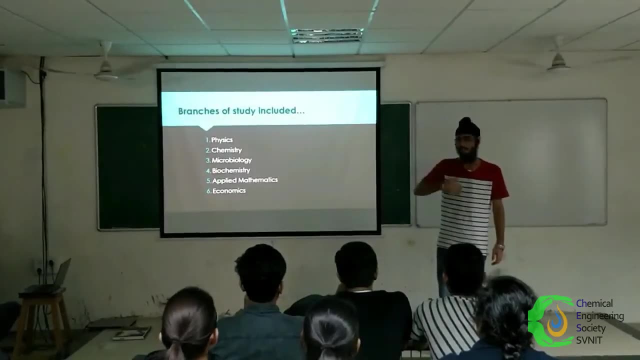 bunch. Only we are taught all the subjects, all the basic sciences like physics, chemistry and maths. No other branch is taught chemical engineering, except chemistry, except us right, And apart from that, microbiology and biochemistry are a part of chemistry. so that is fine. but 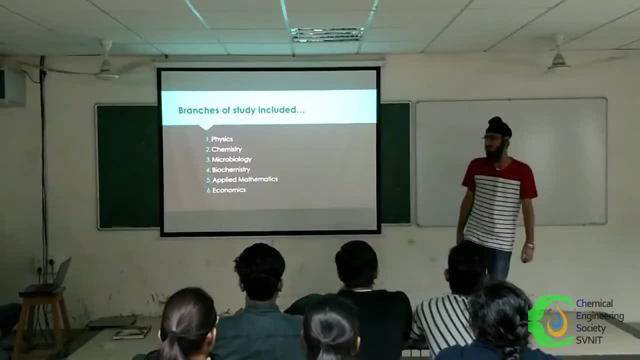 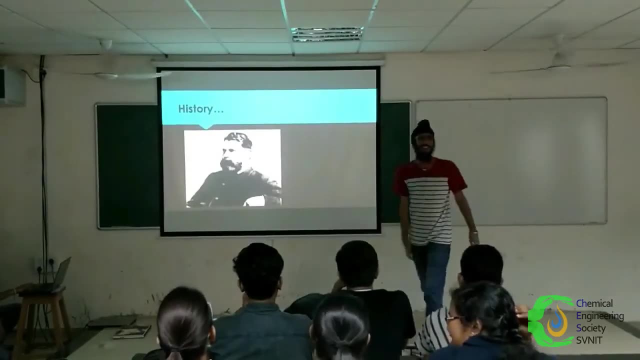 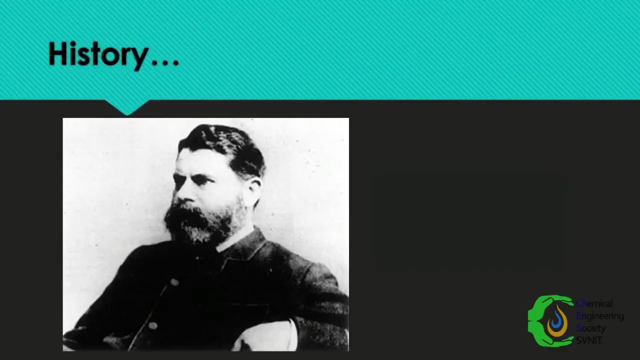 we are also taught economics. So, yeah, you will get to know more about that in the further slides, right, Okay, so I want you to guess who this person is. Hint, this person is known as the father of chemical engineering. 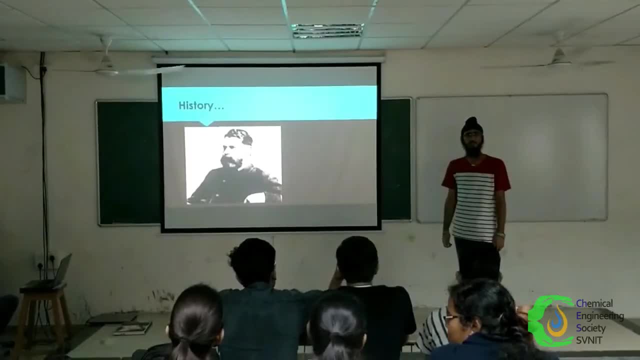 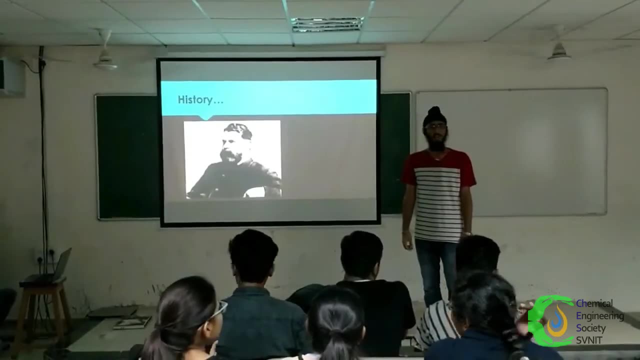 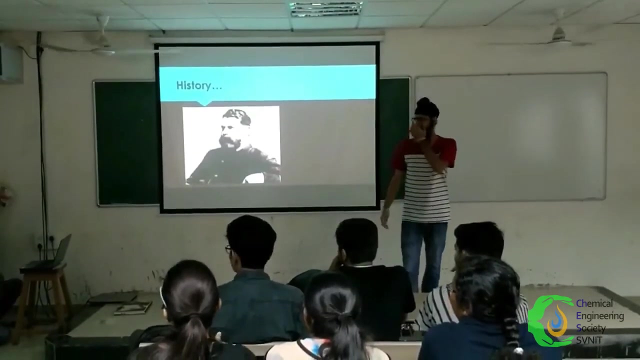 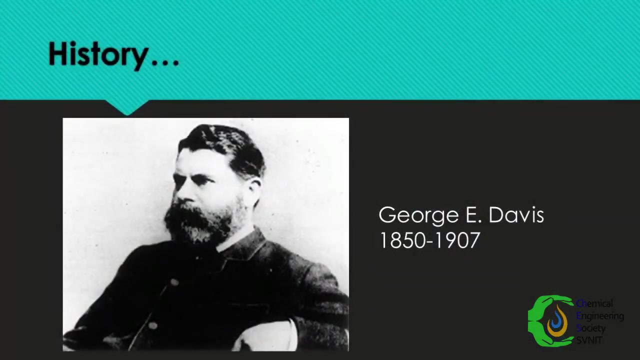 Please raise your hand if you know. okay, Third year. third year, I think you might be knowing. Anyone wants to like give it a guess? No, Okay, fine, I will tell you The person's name is George E Davis. okay, And he is regarded as the father of chemical engineering. 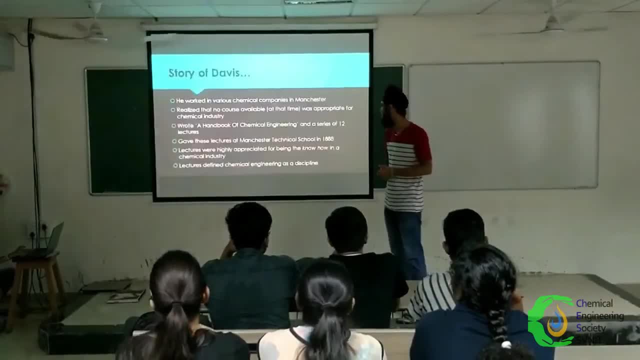 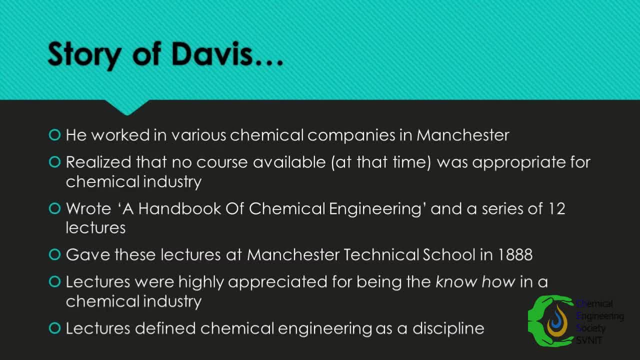 of Davis. In brief, Davis was a chemist who worked in various chemical companies in Manchester in England right, And when he was working there he realized that no branch, no field of study, that is, that was available at that time was sufficient to make you know employees. 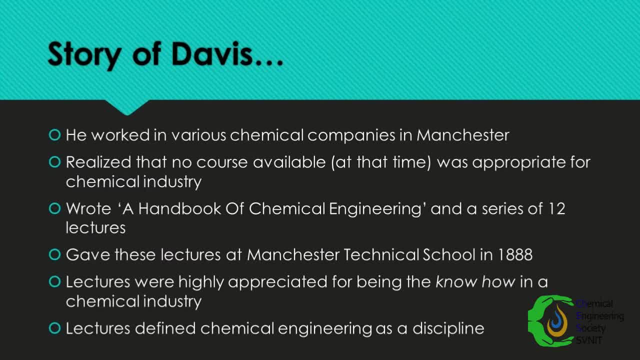 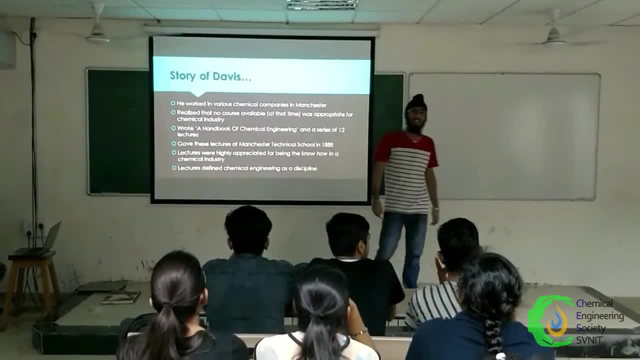 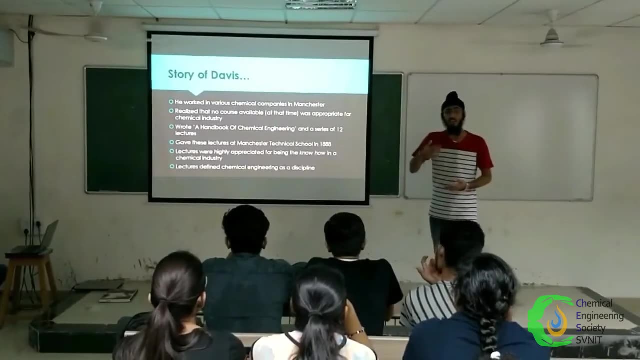 for those chemical companies. So he like, he wrote a handbook of chemical engineering, and this is important. he wrote a series of 12 lectures that he delivered at Manchester Technical School, and these 12 lectures, they became the foundation of what we study today as chemical engineering. 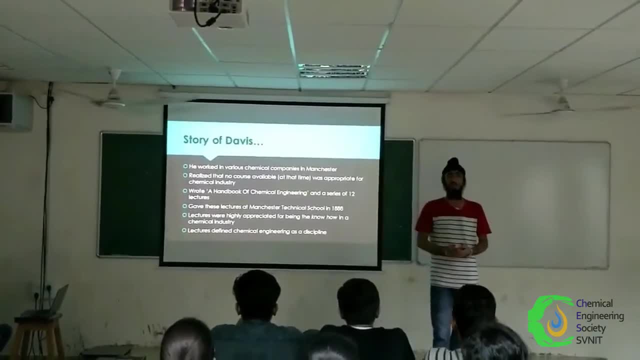 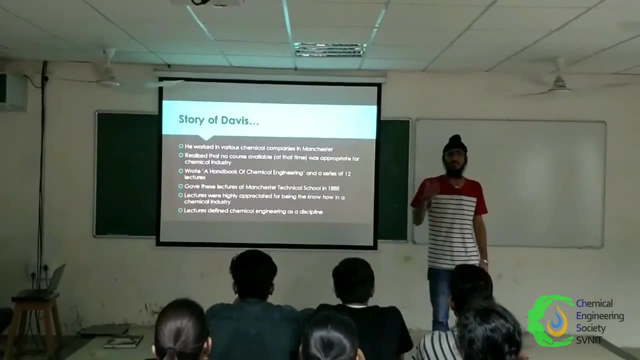 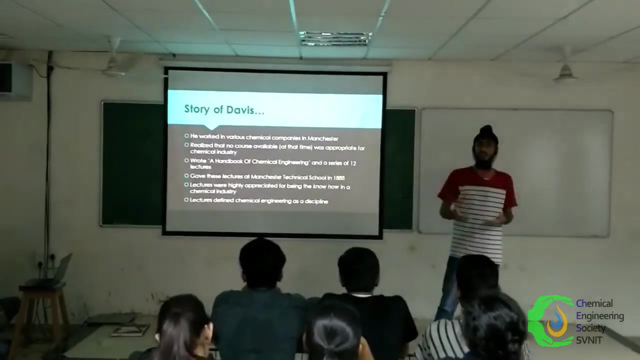 That's why he is regarded as the founding father of chemical engineering and at the earliest level, chemical engineering was meant to be a specialisation of the available courses, like mechanical engineering at that time. It was not meant to be a wholesome course in itself, it was meant to be like a specialisation. 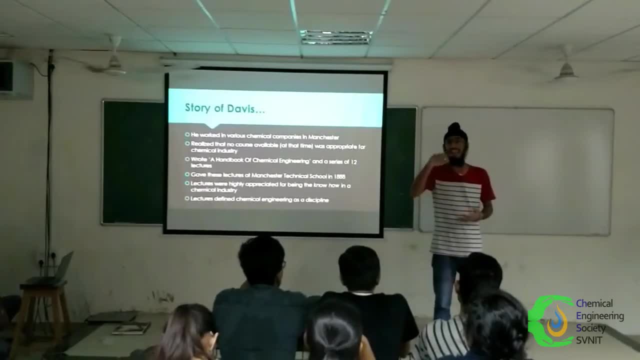 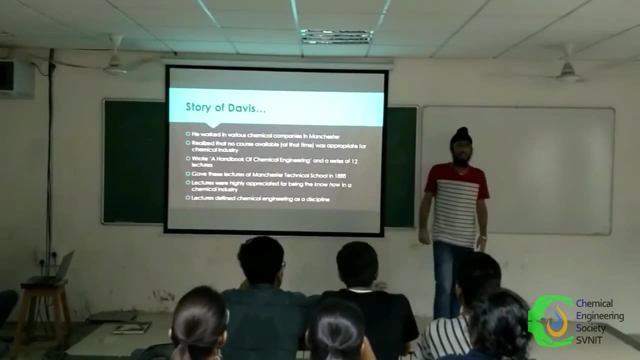 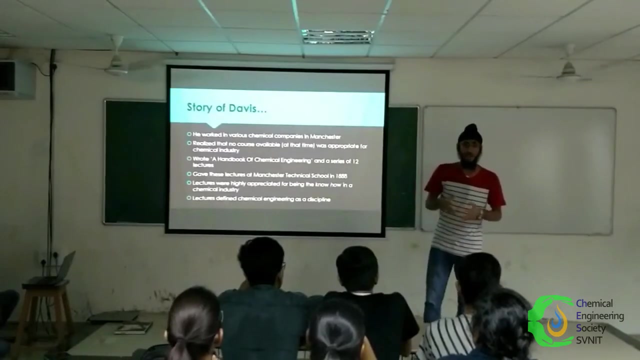 but, like MIT, started a course X for chemical engineering in 1889, just after this year, and it was like a specialisation. it was not a wholesome subject, but soon after developments came in and people realised that it cannot be treated as a specialisation because there 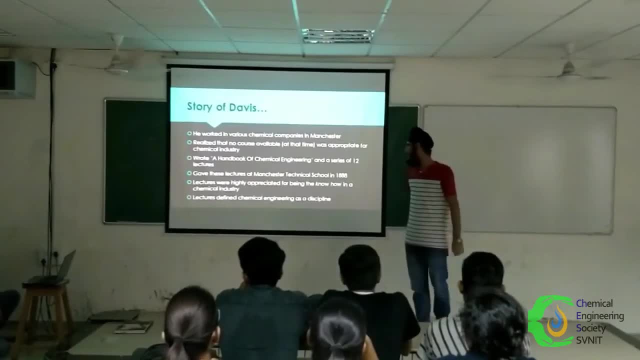 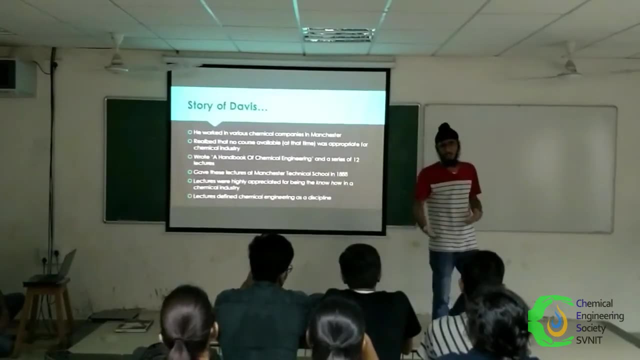 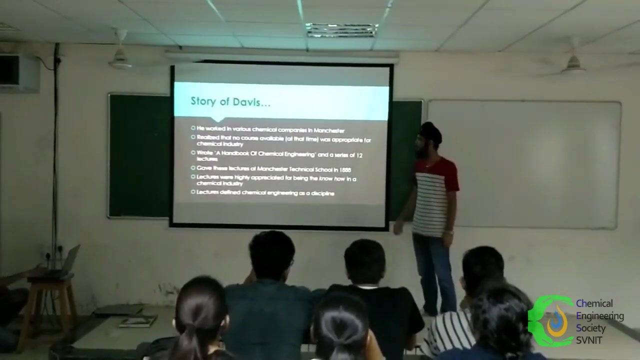 are too many subjects to cover, So they made it interesting. It was a separate branch and today what we study is not exactly the 12 lectures, but it's a modification of those 12 lectures, as well as some developments that were like some inputs put in later. 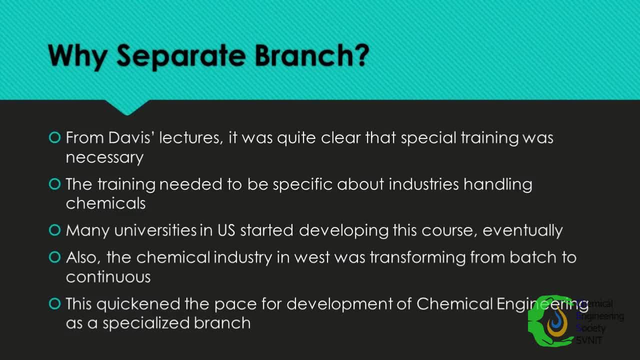 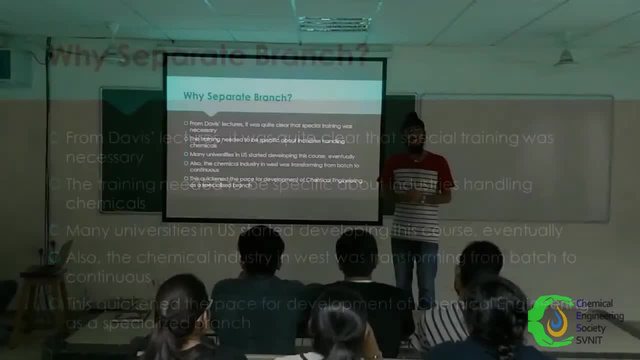 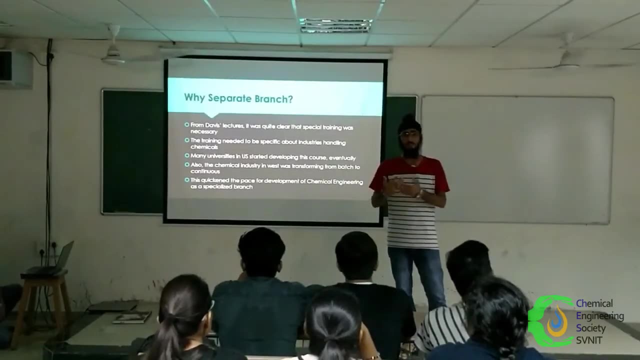 So this is what I just said. it was quite clear that a special training was necessary and the training was required to be specific about companies that handled chemical At that time: mechanical engineers, engineers, engineers, engineers, engineers, engineers, engineers and chemists. they were responsible, considered responsible, for running the plants. 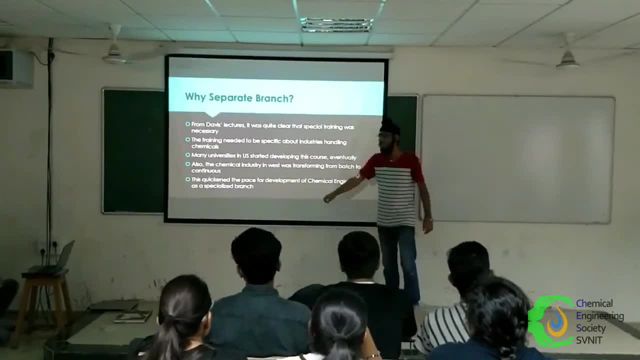 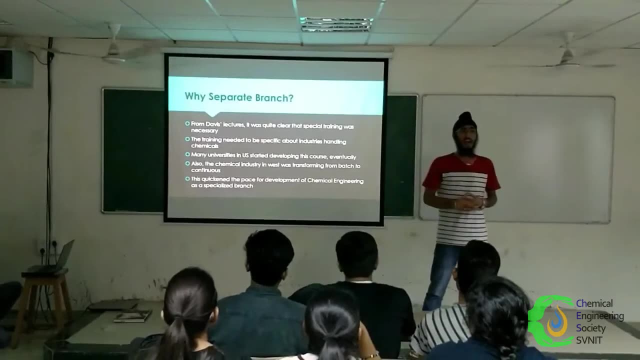 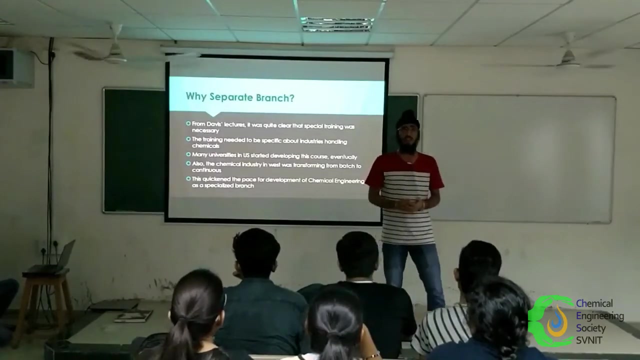 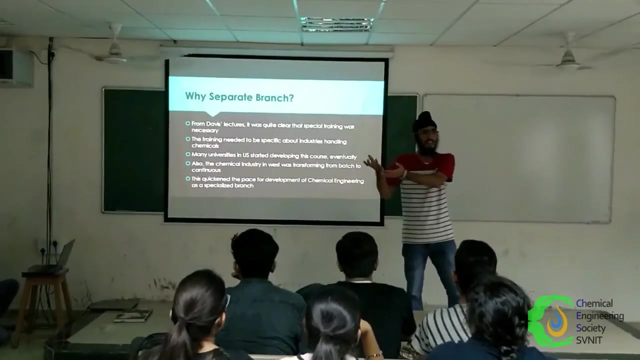 that handled chemical Also. this was the time when industrial revolution in London, or in England as a whole, was just about to begin, and so this gave like a boost to the development of chemical engineering, because people realised that as they shifted from batch processes- second year i guess they know what batch process is right- they shifted to continuous processes. 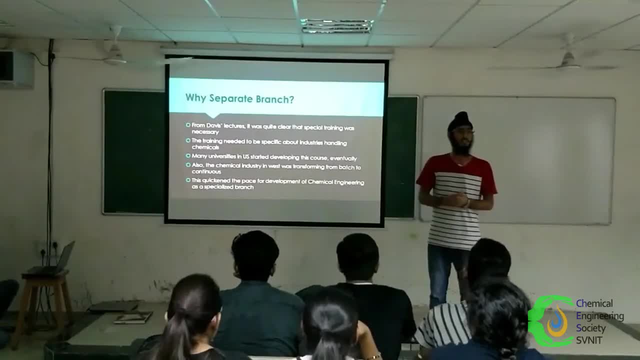 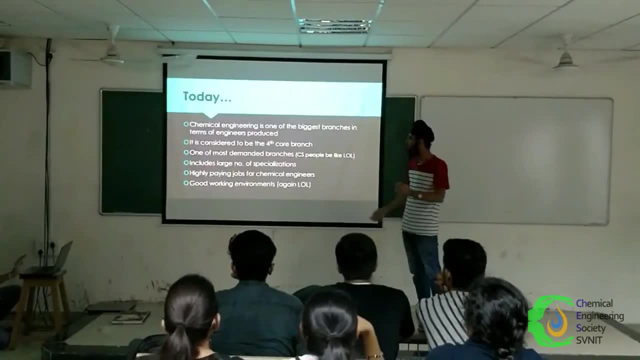 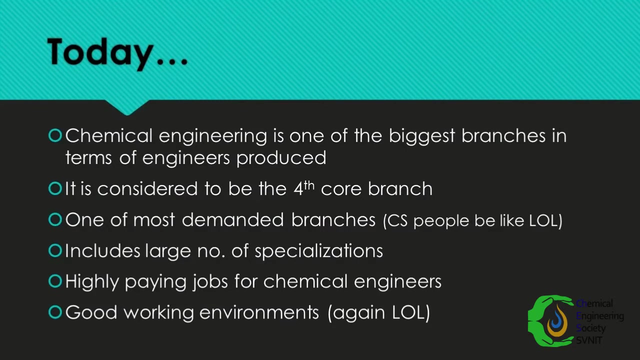 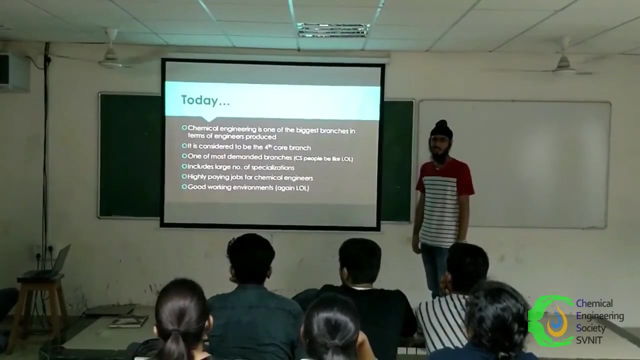 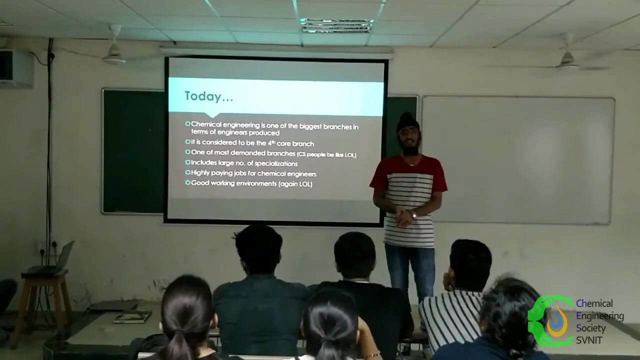 more detailed knowledge about how chemicals behave and all that was necessary, and today it is one of the biggest like brands in terms of engineers produced and, well, one of the most demanded branches. but not in the context of india, uh, in western countries, to be precise, us and canada, i think it is one of the most demanded branches because of 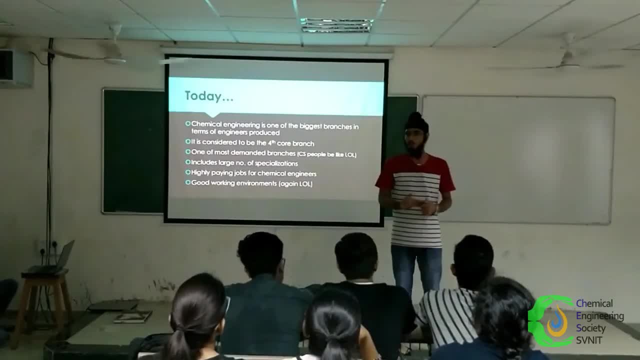 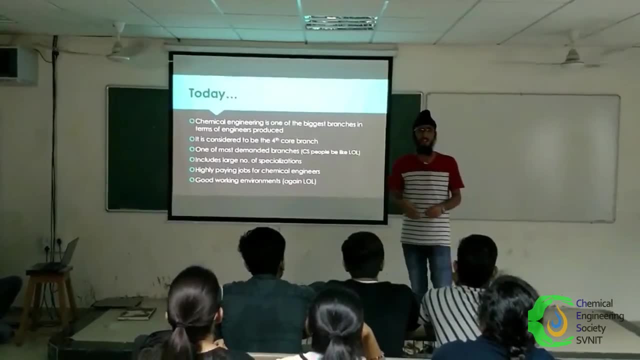 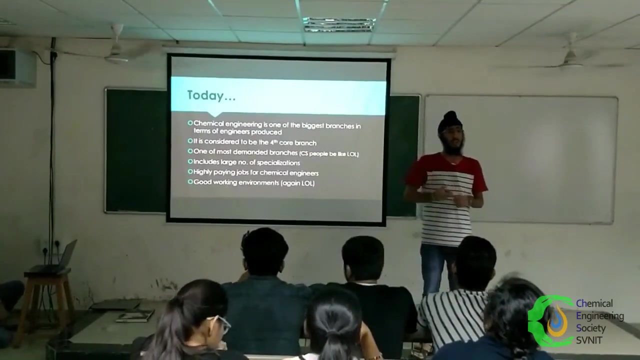 uh, technology, shale gas technology, you'll come to know about it. shale gas technology is like a recent development in the field of petrochemicals and petroleum engineering. so, and shale gas, shale gas technology was recently like invented. i can, uh, i can say in us, and so for that reason, 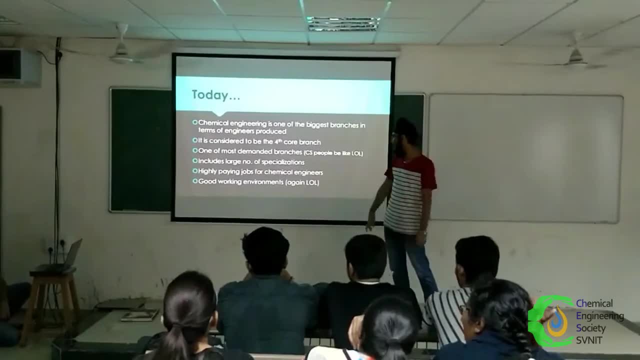 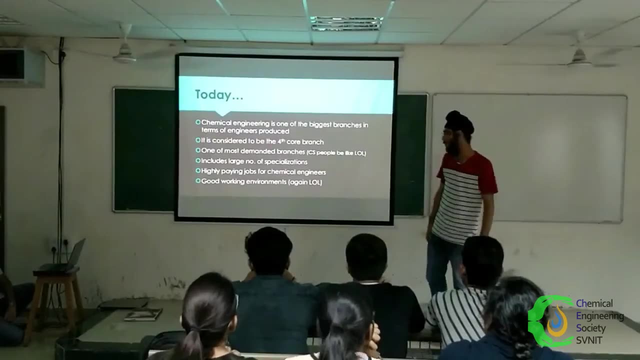 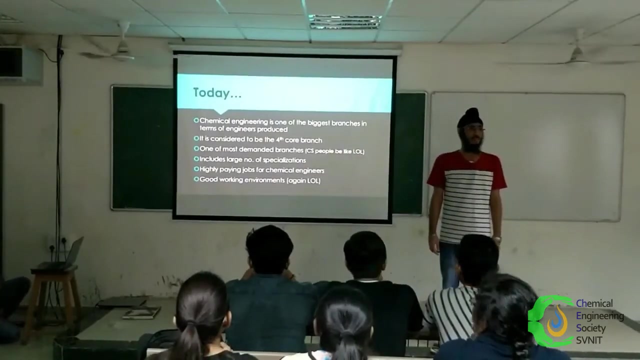 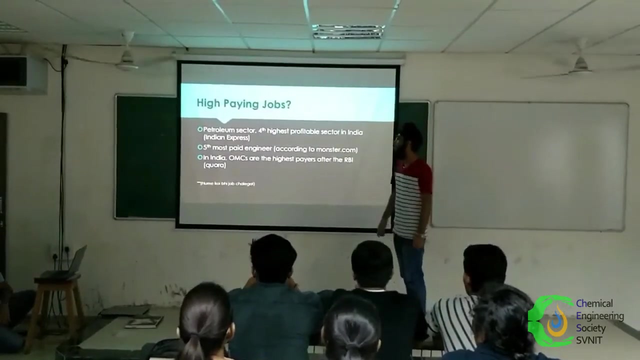 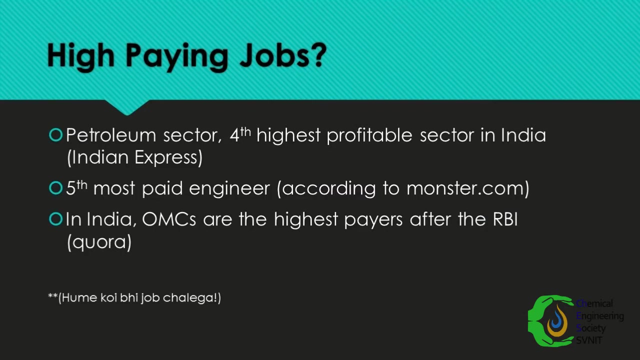 chemical engineering is quite in demand over there, right, and high, uh, like high paying jobs. if you are thinking high paying jobs, so i'll tell you why. good working environments, right, okay, so this is why they are high paying jobs. and the- i have included all the sources. uh, this point, see, i cannot like take responsibility. 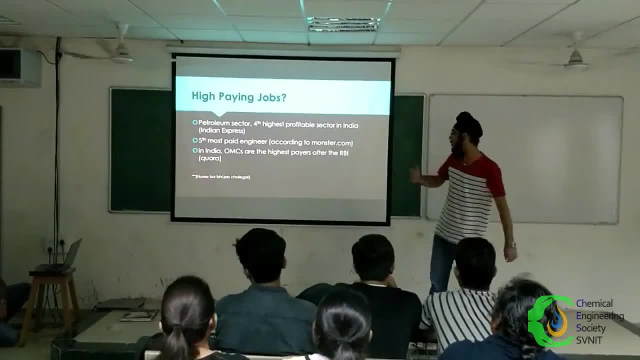 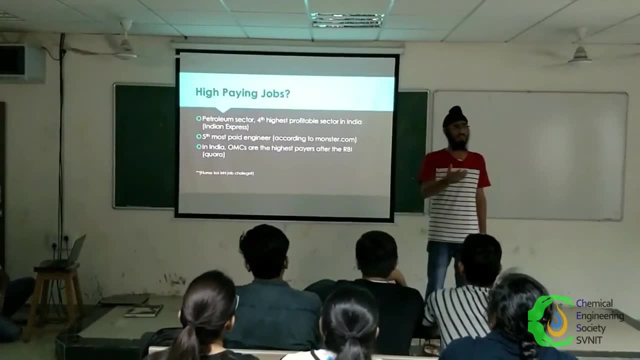 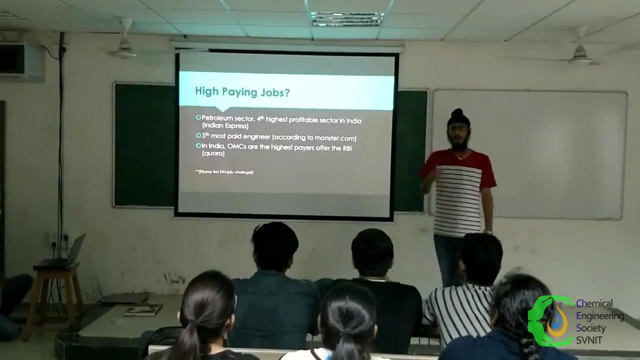 if this is wrong, because i've taken it from quora and then the person had answered that after the rbi posts, after rbi omc's- you know what is omc? anyone omc third year omc's what? oil marketing companies? oil marketing companies. currently. do you know which is the biggest psu in india? iocl. iocl is the biggest psu and it is the biggest pair in india, or it is the highest recruiter of chemical engineers in india. in india, right now, this is the biggest psu in india. i think that european chemical 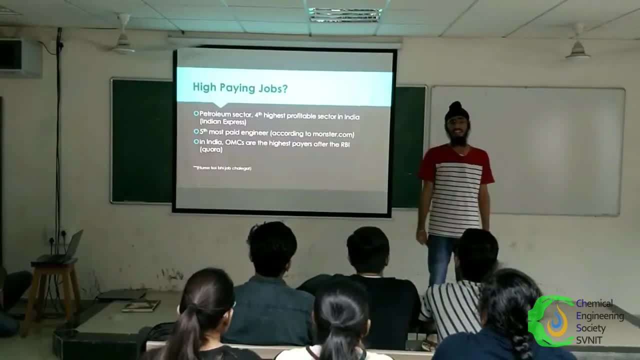 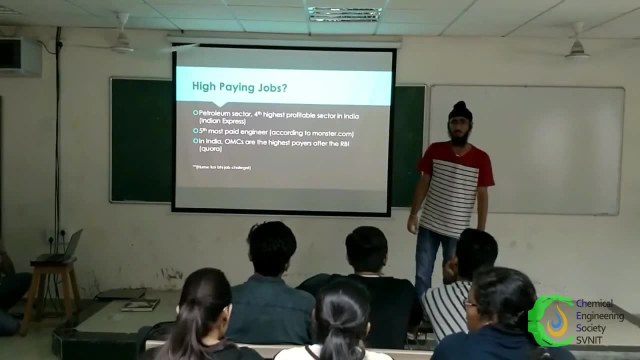 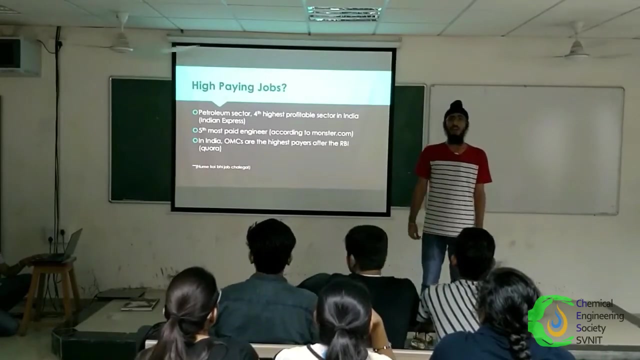 engineers and iocl is very big right, uh, uh, beginner beginner packages: 14.5 to 15 lakhs- okay, and 1 year later nearly 20 lakhs reaches per annum- okay. and the other csit guys also earn good, obviously, no doubt, but their uh, lifetime of job is very less. we are 60 years old, so we are. 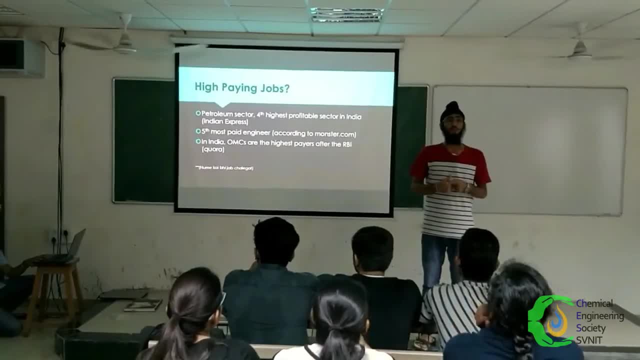 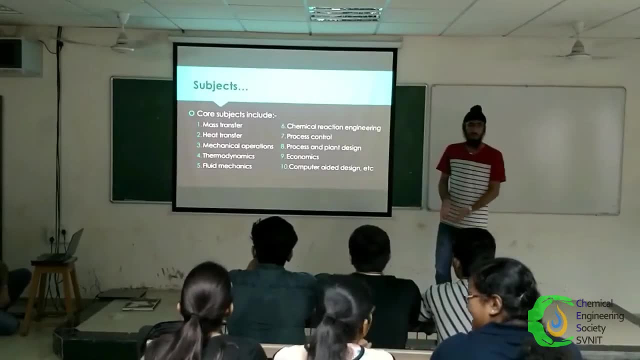 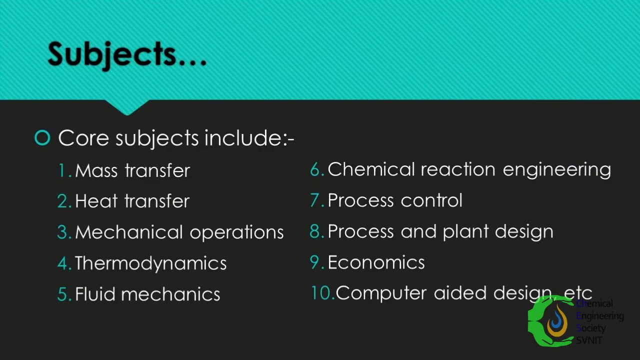 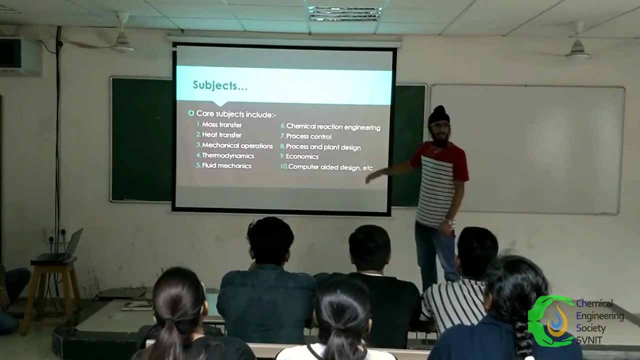 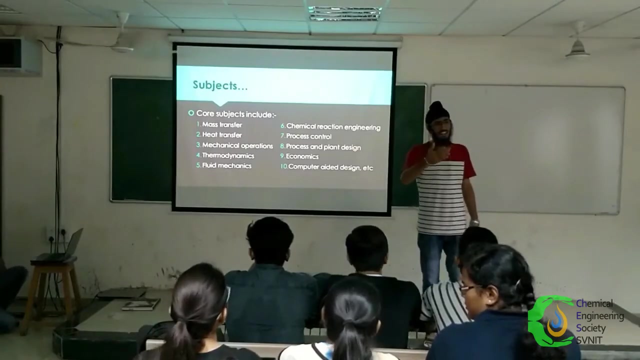 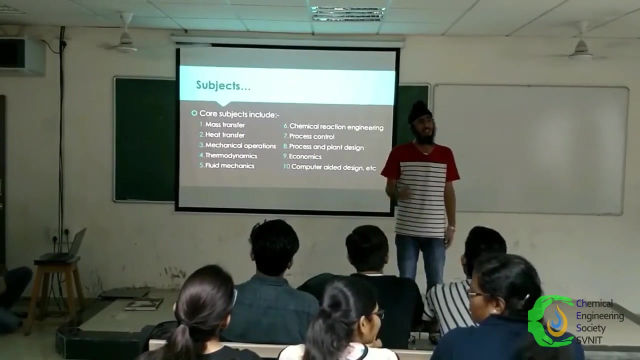 60 years old. right on those days try to come out and say: we are doing well, okay, yeah, okay, So okay. now coming to subjects. these are not all the subjects. these are the important subjects that you will cover. core subjects: second year mein ek bhi nahi hai, ek hai PC hai, GCT hai aur materials hai, but usme maza nahi aata hai process calculation. abhi akli semester mein aayega tume tike. so second year mein, like second year ka problem hi hai. this is why we arrange this orientation, because after second year no one has an idea what chemical engineering is. 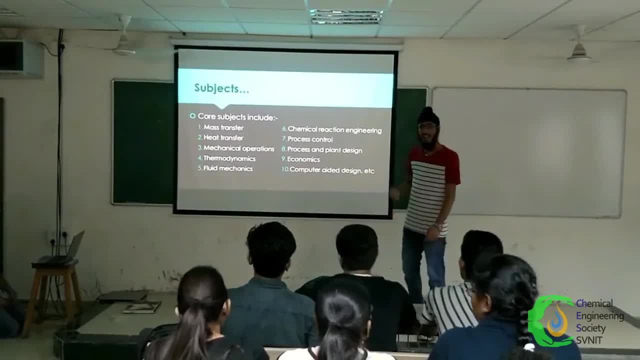 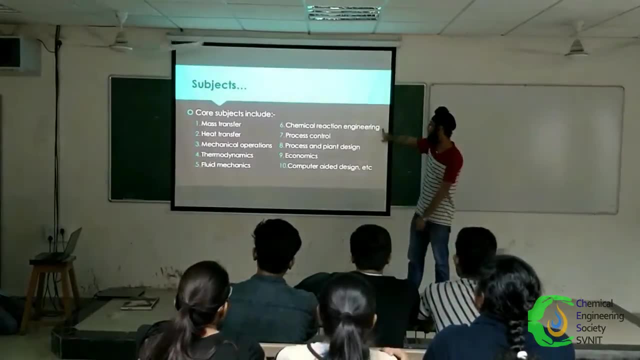 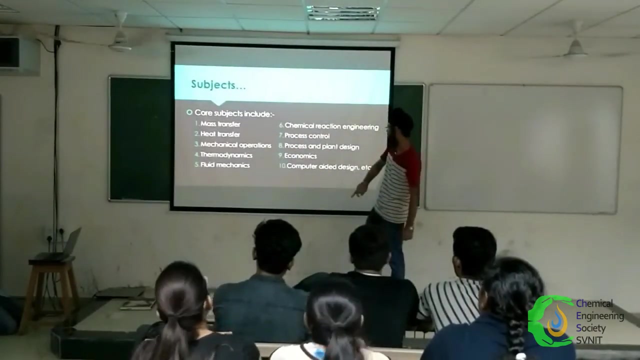 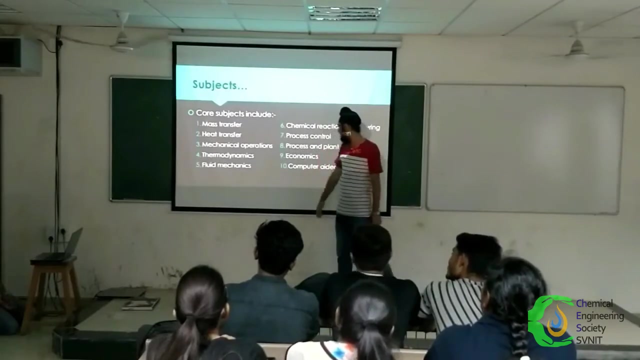 do saal ho jaate hain. amko pata nahi chalda. chemical engineering mein hai kya tike. that's why we arrange this aur fir. these are the important subjects. ha to mai kya bolata. chemistry sirf is subject mein kaam. aati hai physics, physics, physics, physics, bas tike mechanical operations, mein thodi baat physics lag jaati hai tike fluid mein bola yaar. 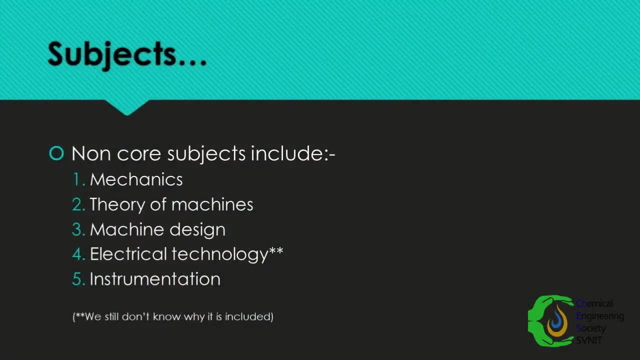 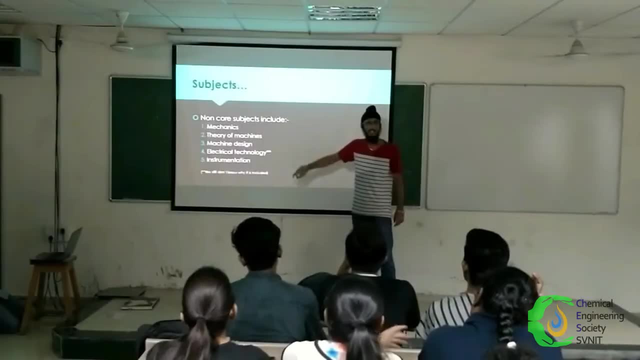 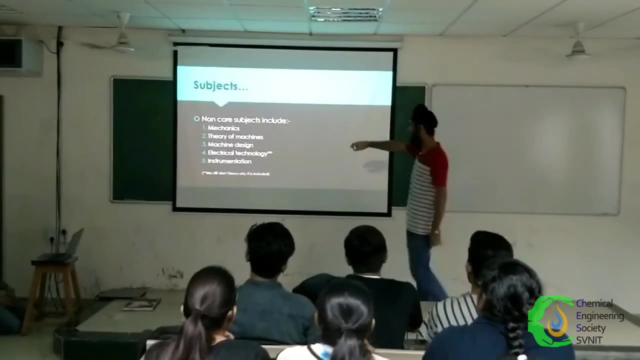 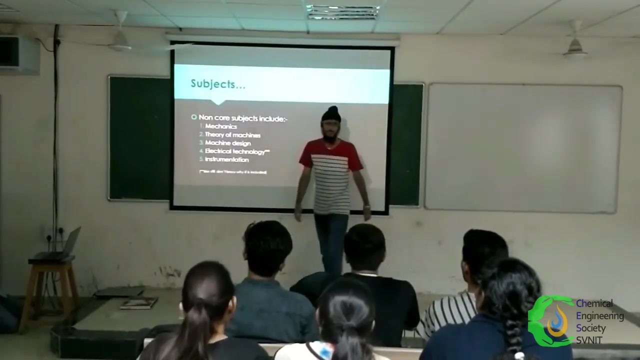 this is. this is yeah. coming to non-core subjects, second year, poora bhar hua hi hone se specialist mechanics, then theory of machines. agal se tercer mein aega KDMI main subject hai: theory of machines and machine design. ok, so these 2 are subject, even though they are not the core subjects, but these 2 subjects are important. ok, these 2 subjects, and even solid mechanics is also like. it's fine, thoda bohot aa jaayega use mein. 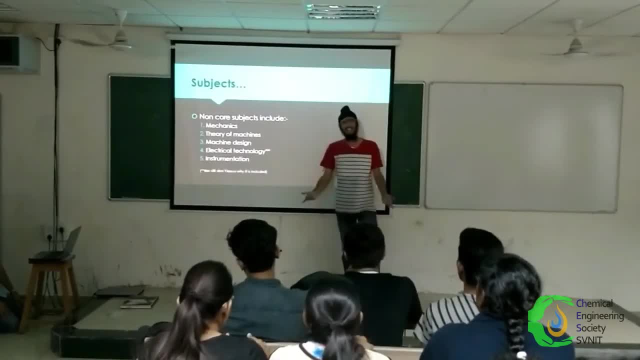 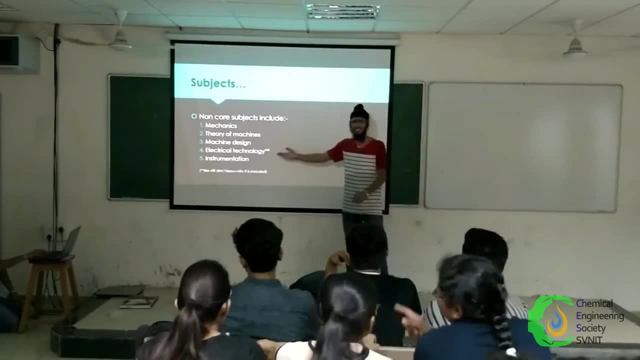 but yeh subject toh. kyu hi hai understand beep dogs meen. Why is this subject important? I don't know. Instrumentation comes in our final year. I don't know why it is mentioned. We don't do anything about it. 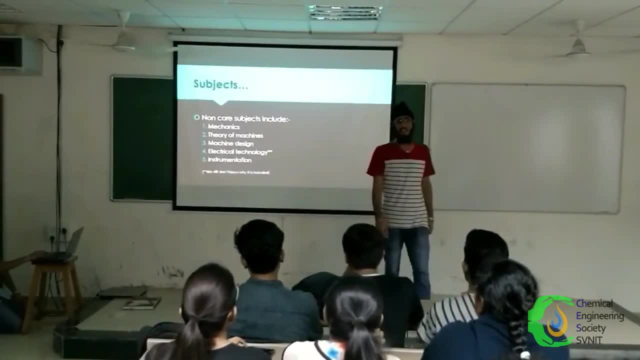 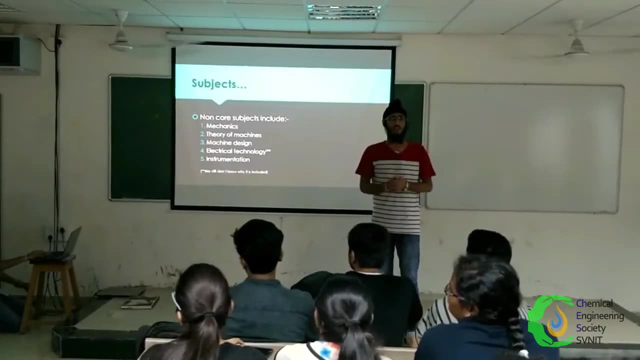 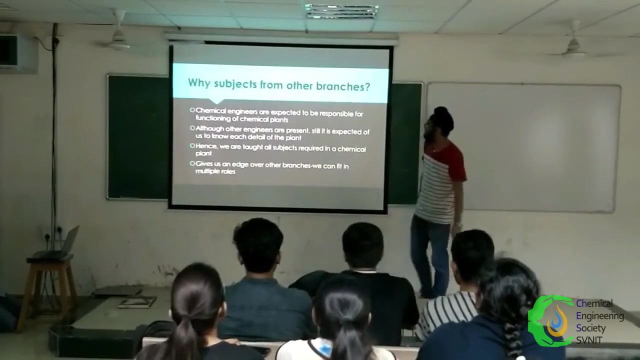 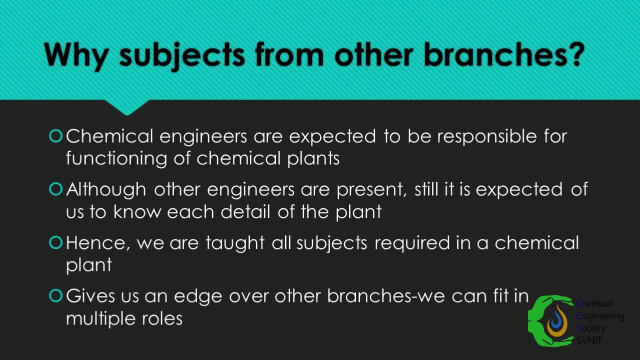 Instrumentation is an important subject. Even though it is in non-core, it has vast applications. Vast applications when you pass out and go to a process control industry. Okay. so this is why we are taught subjects from other branches, The reason being that we are expected to be responsible for running of a chemical plant. 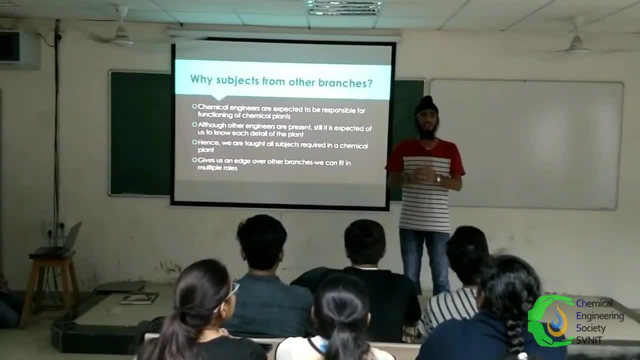 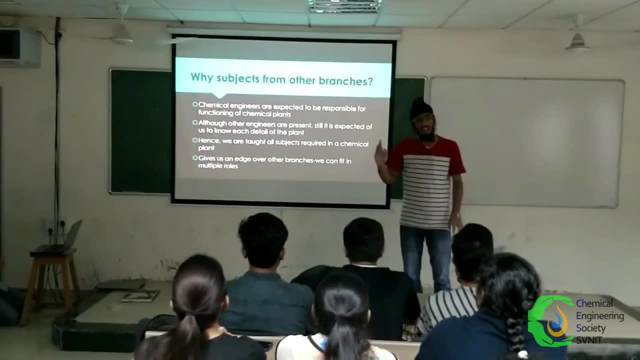 For a continuous process plant, And there we are expected that we should know everything about that plant, Ranging from pumps, motors, transformers, everything. That's why we are taught these subjects, But the thing is, today this concept has become obsolete. 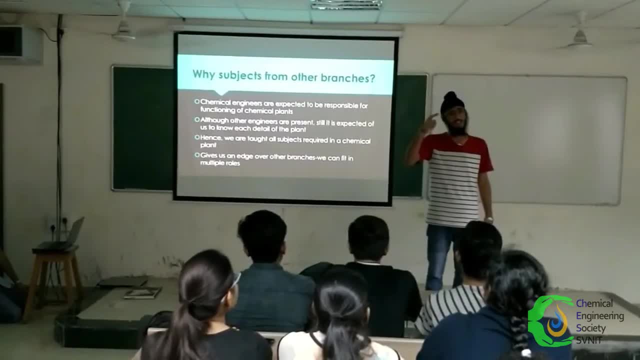 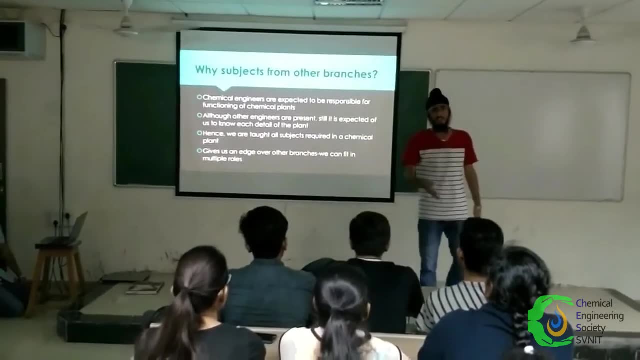 Today, if IOCL is hiring a chemical engineer, then IOCL electrical or mechanical engineering is also being hired. We don't need to do these functions. We don't need to perform maintenance of pumps and all that. Mechanical engineers are there for that. 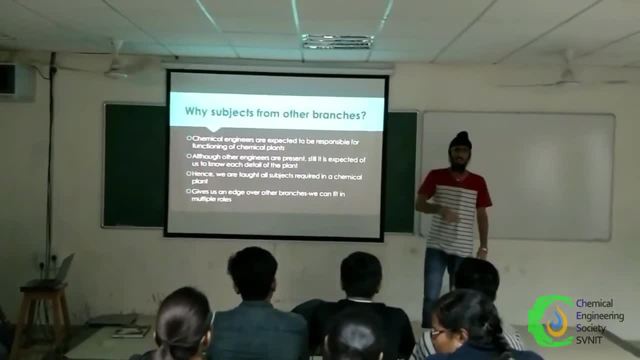 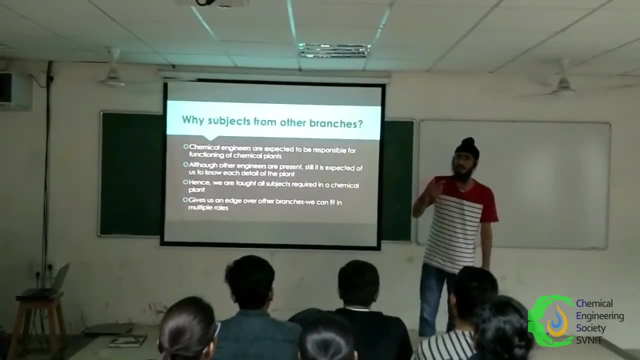 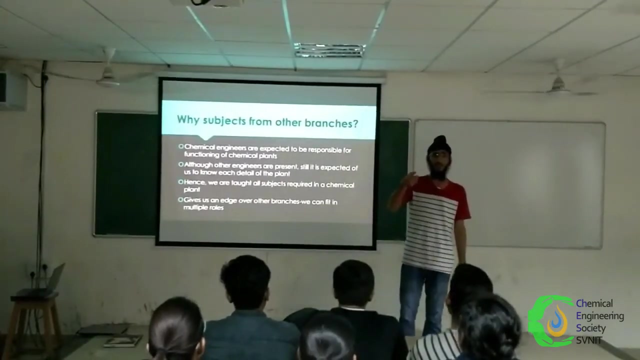 But still this was the basic reason why those subjects were included. Recently, a lot of efforts have been made to change the syllabus. Like, economics is a subject It is being planned to be introduced in second year syllabus. However, due to It is a government college, 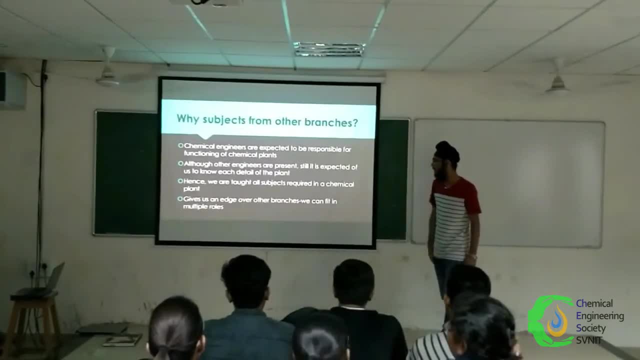 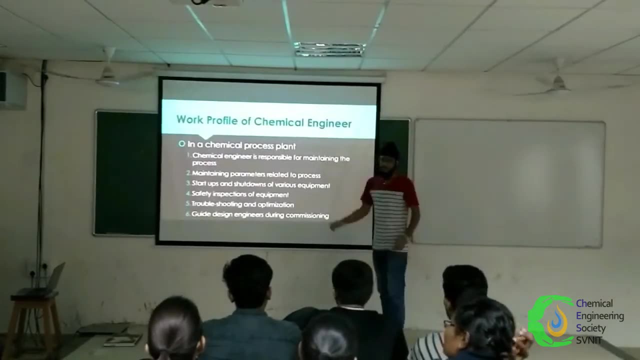 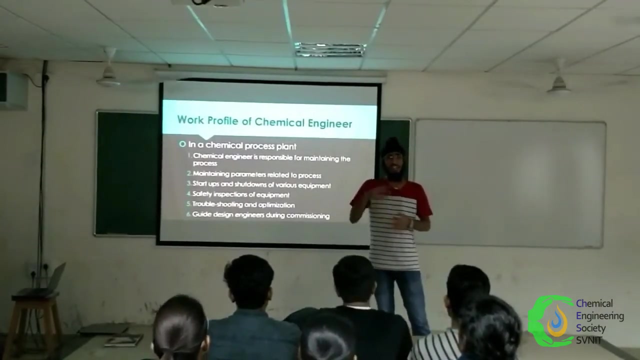 So nothing happens. Everything goes slowly. Okay, so what is the work profile of a chemical engineer In a Okay so engineer is? If you want to join a technical field, then there are three main fields, sub-fields for that. 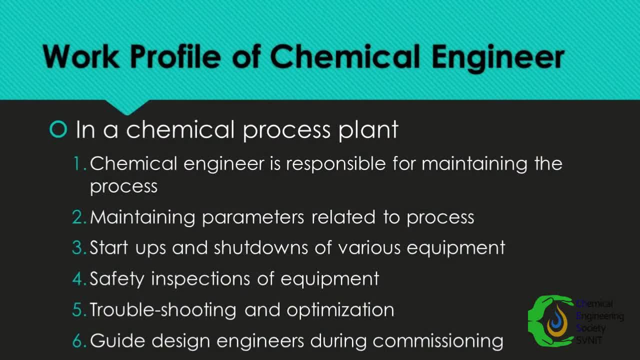 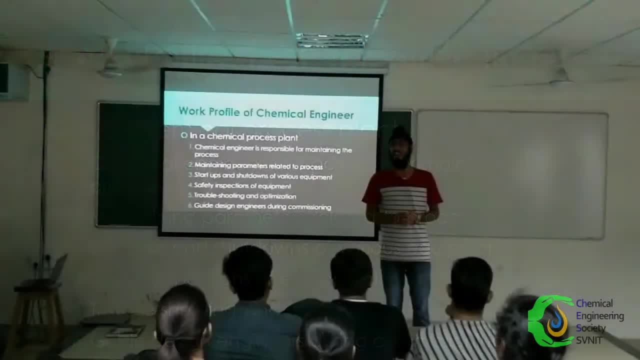 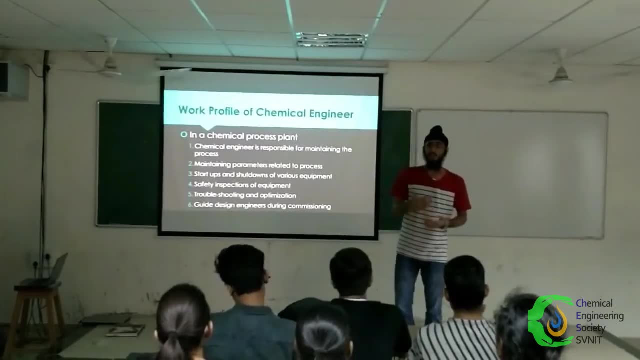 One is chemical process plant, One is research And one is design. So in chemical process plant you are like responsible for, as I said, running the chemical plant. You are responsible for seeing that the processes that are happening, they do not go like in a haphazard manner. 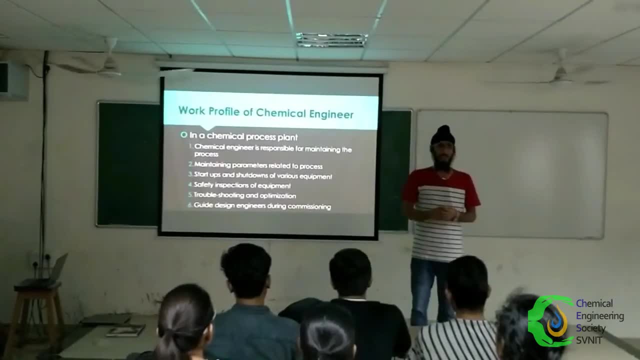 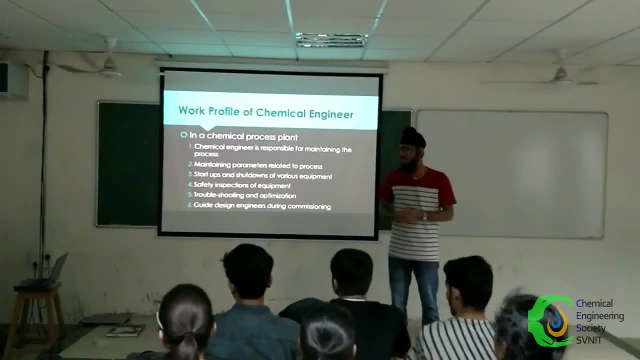 They remain on the way that they are designed to be. The basic thing is you have to sit on a control panel. You have to see temperature, pressure or flow rate. There are three parameters: Temperature, pressure, flow rate. We just have to see this. 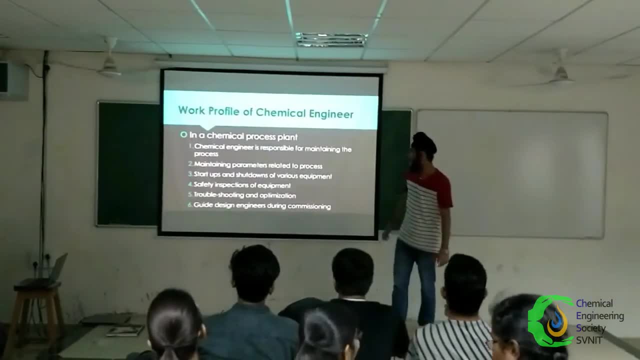 Nothing else happens. I am telling the truth. the work of a chemical engineer in a chemical process plant is only done at this point, only when the start up has to be shut down. Otherwise they sit like this only If someone has done an internship in third year. 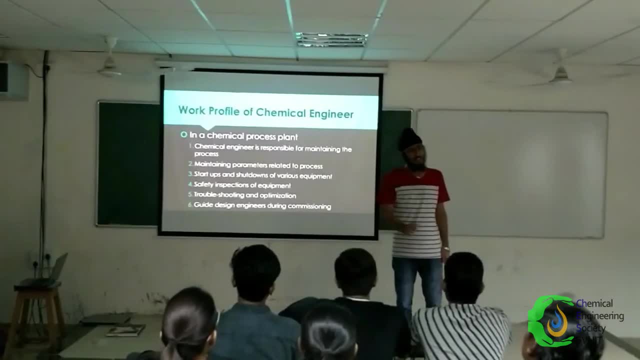 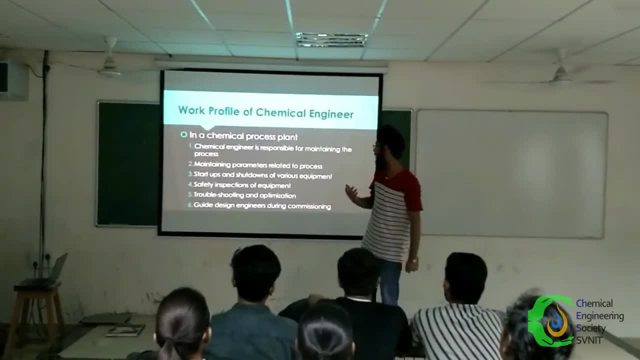 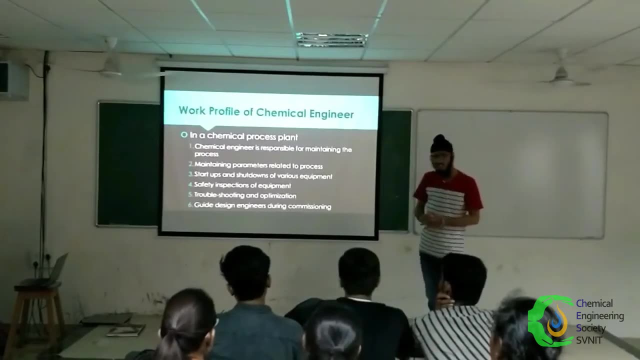 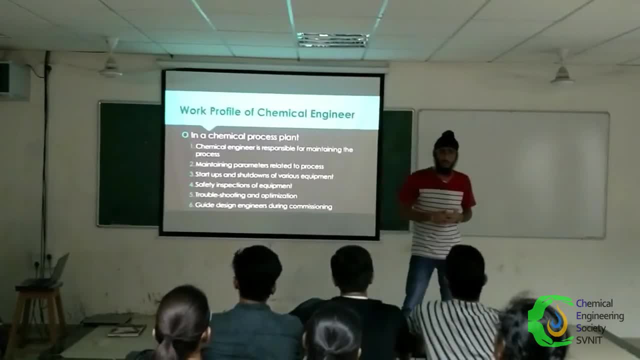 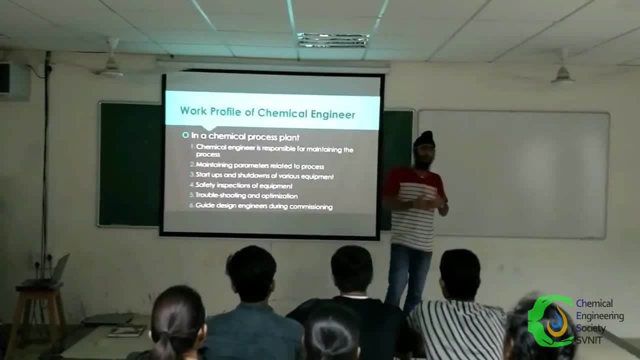 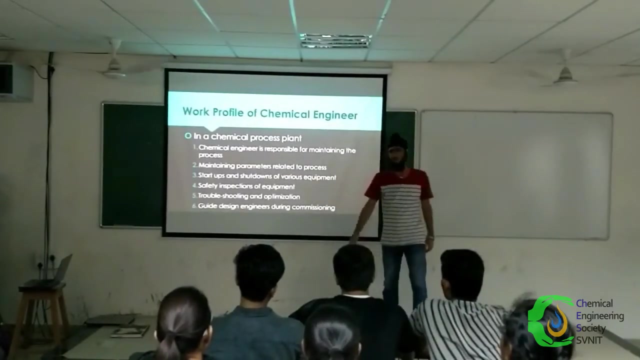 is not giving as much efficiency as it is designed to give, then they have to troubleshoot. Troubleshoot is basically finding what the problem is, And optimization is after the problem has been identified. you have to rectify the problem. So this is like small portion of their job. 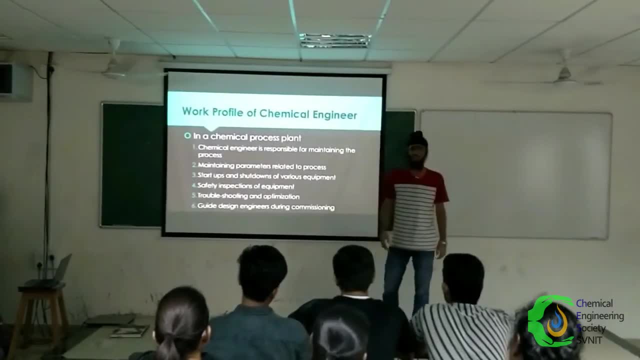 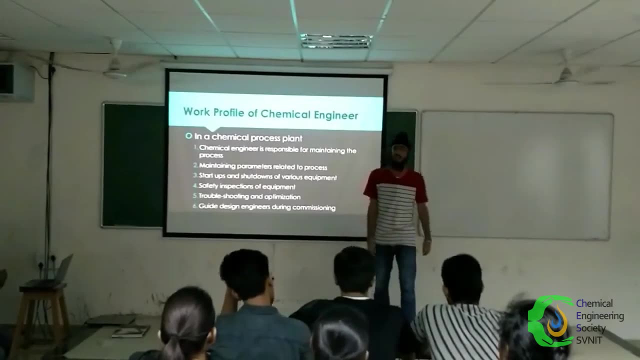 And you get a lot of money in commissioning. In commissioning the design engineers, we have to take care of them, We have to guide them, Nothing. So this is the most sought after job if you want to go in a technical field. 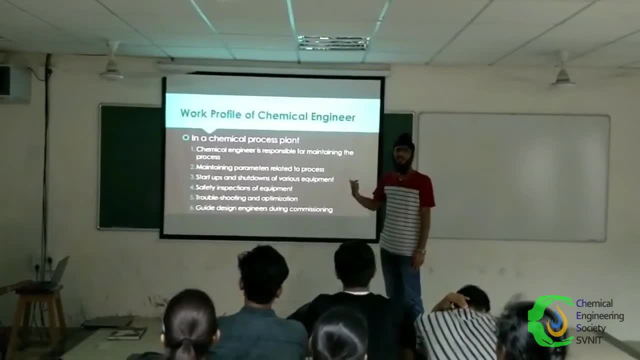 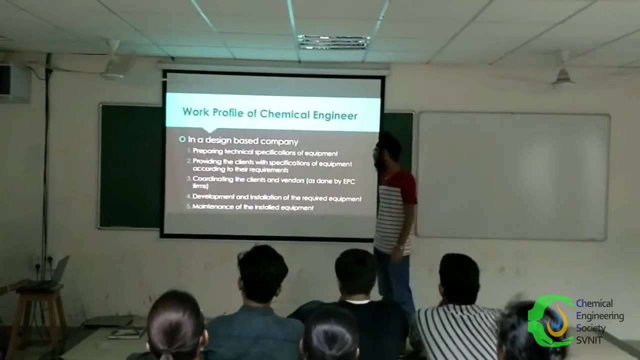 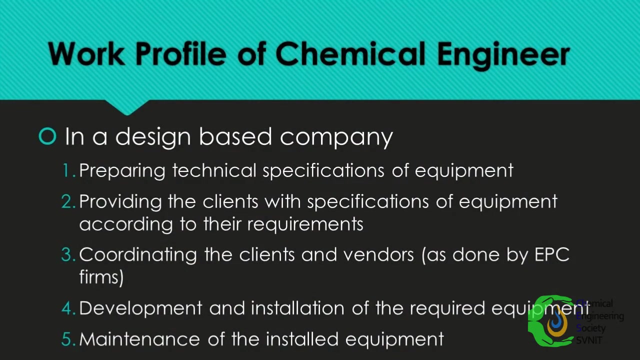 People die for getting jobs in these, in Reliance, these three OMCs- IOCL, BPCL, HPCL- you have to do this, only Nothing is different. This is for design engineers. Design engineers, work is a bit more like complicated. 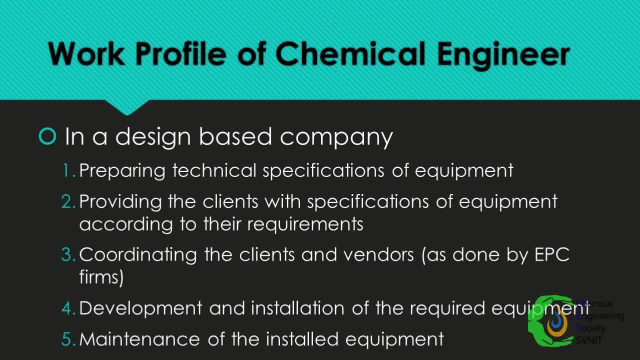 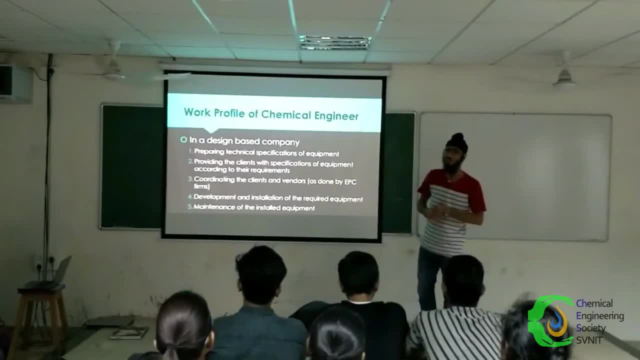 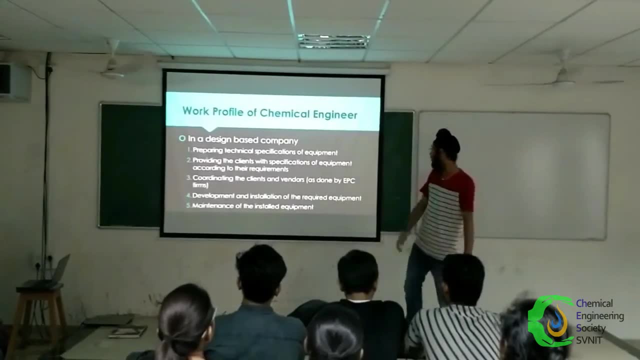 than the process engineers They have to like. this is an office job. by the way, This is not a field job. You have to make technical specifications of a product. You have to deal with clients and prepare specifications according to their requirements, If you. 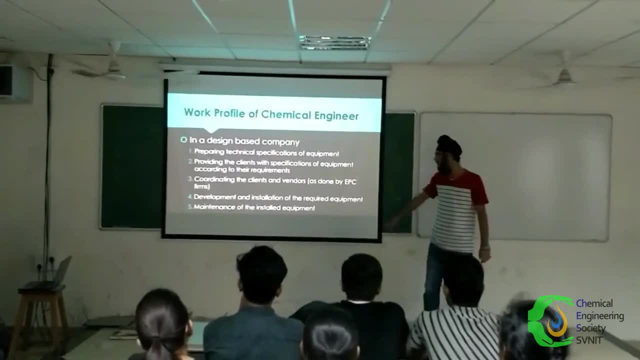 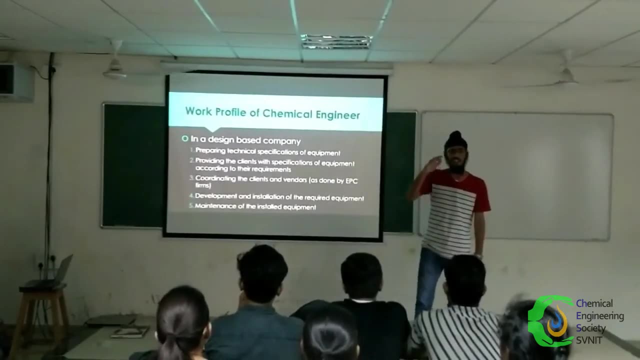 okay, anybody can tell me what is an EPC firm, EPC? EPC stands for Engineering, Procurement and Consultancy. Okay, has anyone heard of EIL, EIL, Third year EIL, EIL Engineers India Limited. 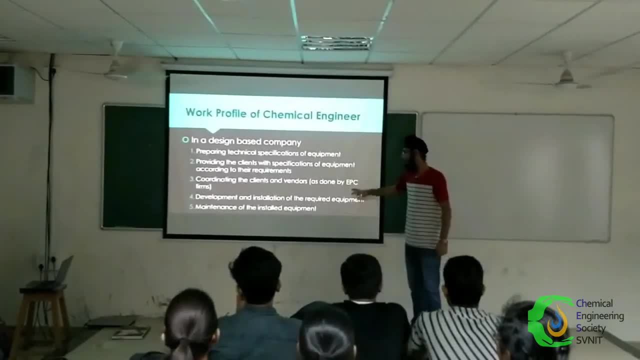 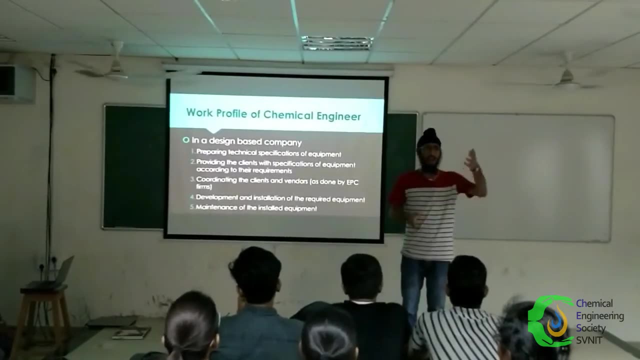 So EIL is one of the EPC firms. that is a PSU, It is an EPC firm. The work of an EPC is basically like. I will give you an example. If take IOCL, IOCL, it requires to install a distillation column. 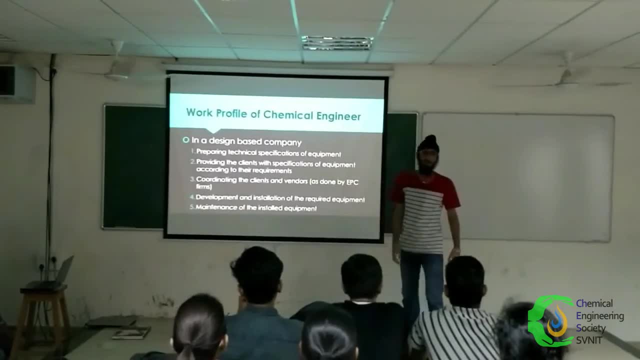 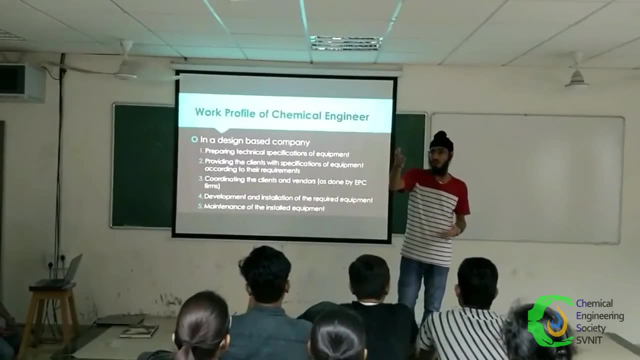 Okay, So they will contact an EPC firm that we have to make this distillation column. The EPC firm will contact the vendors- licensors- you must have studied in GCT. Okay, They will contact the vendors and tell them that these are the specifications. 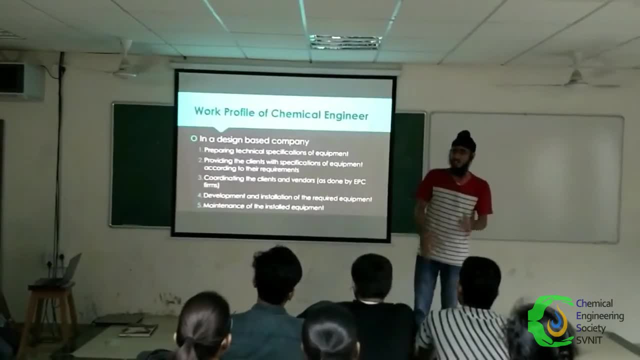 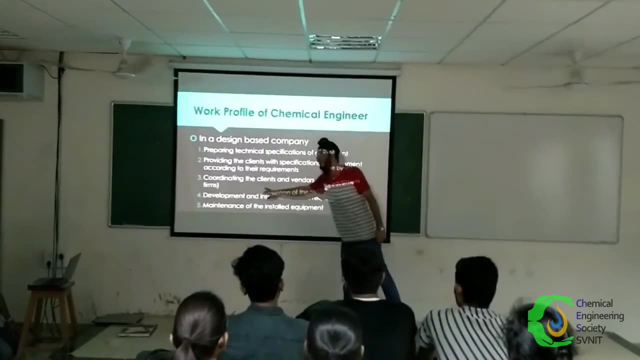 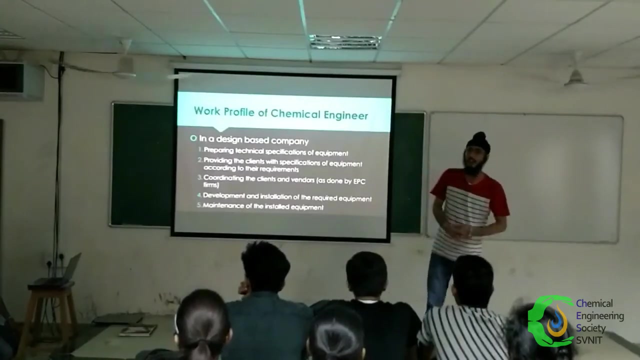 We need this and that for its design. The vendors will provide the detailed specifications as well as the cost. So basically, it is coordinating the clients and the vendors. Nothing else, Right? So this is also like a demanding job, because it demands you to be present all the time. 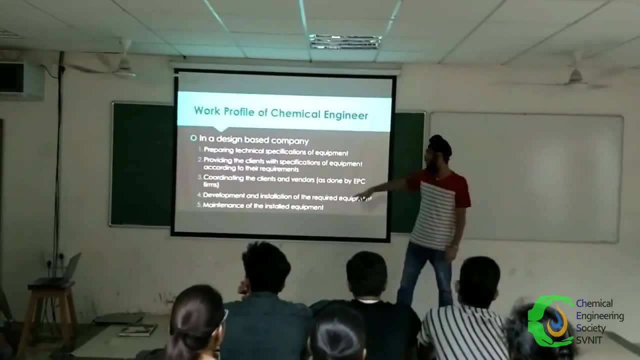 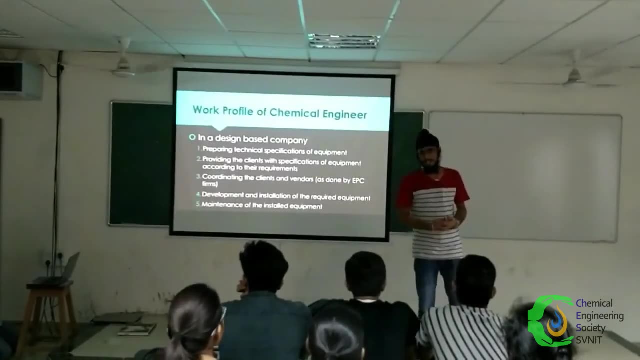 The reason for this is that in India generally, the vendors are foreign companies Like Halder, Topso, Kellogg. these are all companies and vendors And you will study this in the next semester. GCT is a subject in which all this comes. 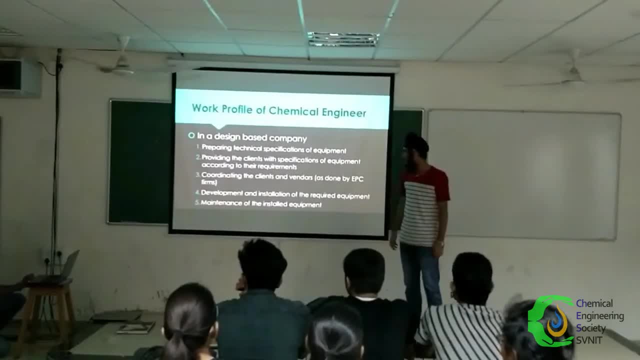 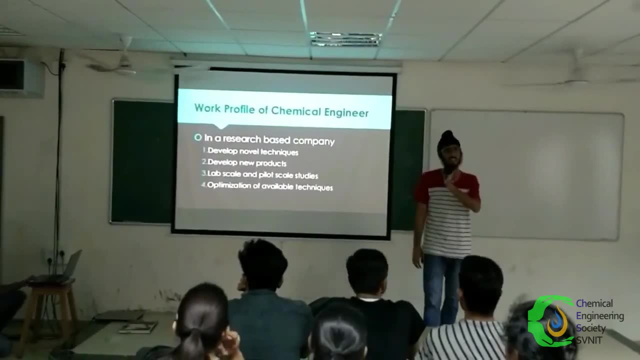 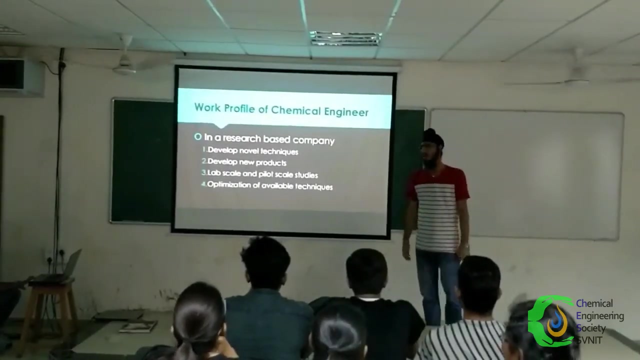 Okay. And then development and installation. all this You have to do. maintenance, Okay, Okay for research. research is like you can only do what you are interested in, Because if you don't have interest in research, 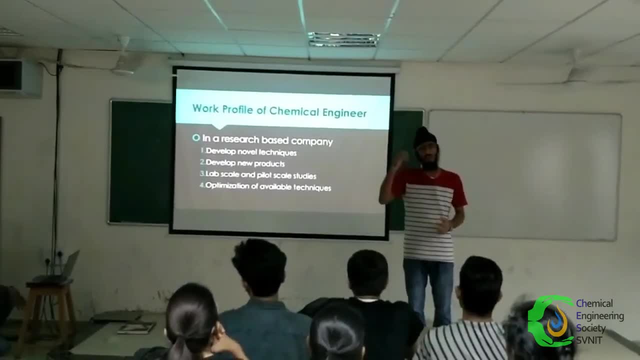 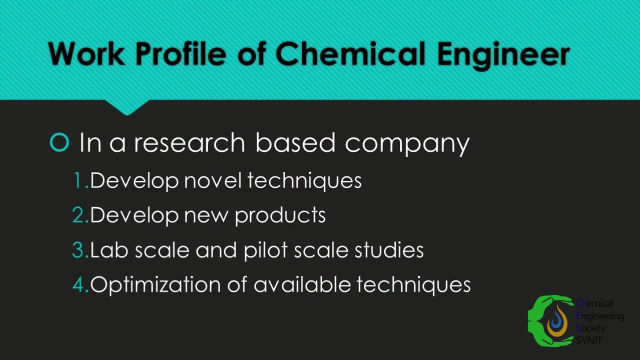 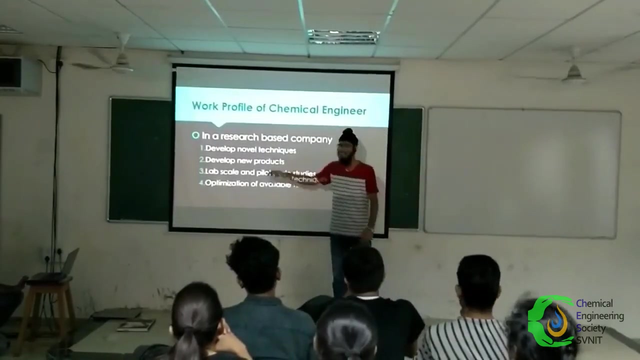 then you will get frustrated Because you have to commit everything to the research. Research includes novel techniques. Do you know what novel means? Novel, yes, Novel, as in something which is more advanced, a little new. So novel techniques of some distillation. 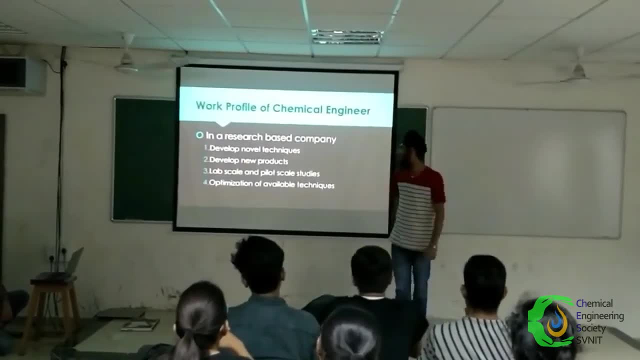 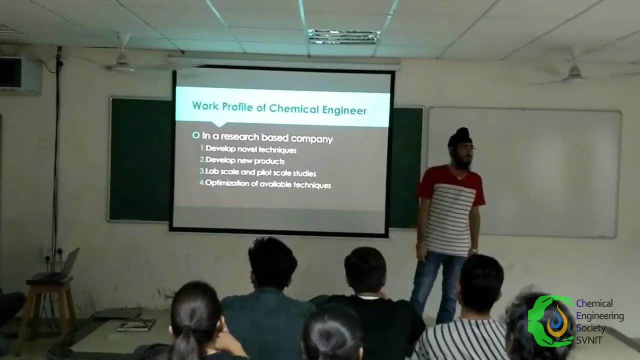 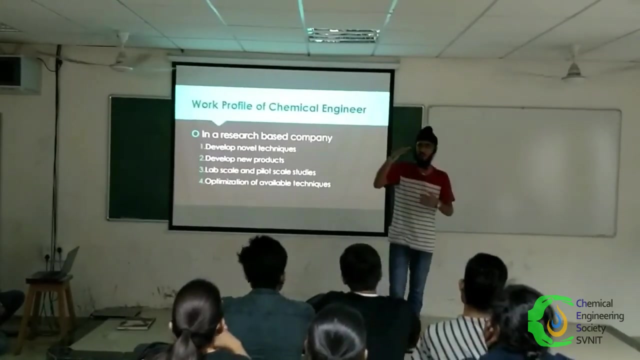 novel techniques of heat extraction. all that Then developing new products. Yes, what are pilot studies? Small scale, but larger than lab scale. Pilot studies is what happens first when a process is developed. how does it work? Its procedure is: 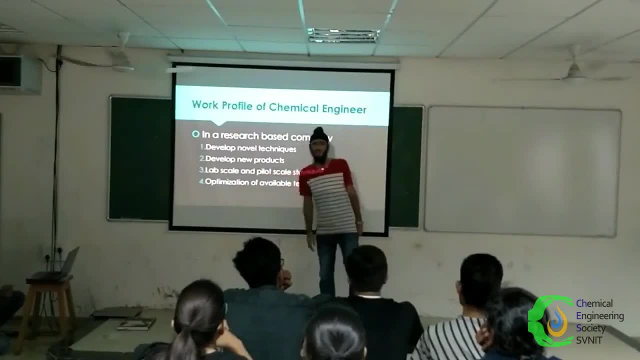 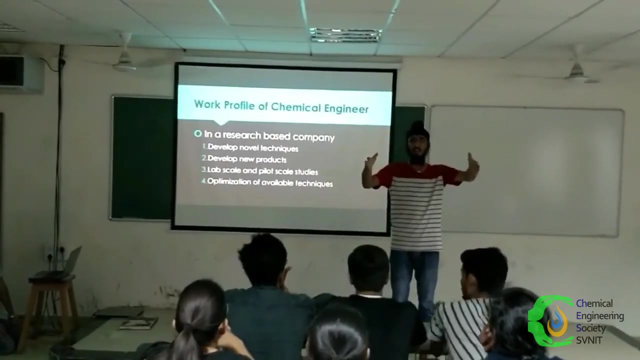 first of all, the chemists work on lab scale. They see that the compound is coming out to be fruitful and the process is good. Then they send the project to pilot scale studies. Pilot scale studies is like we will plant a small plant. 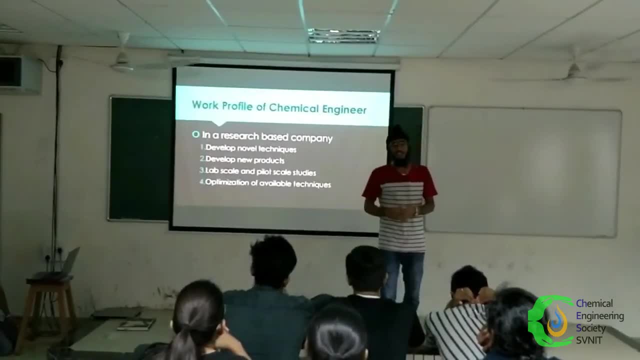 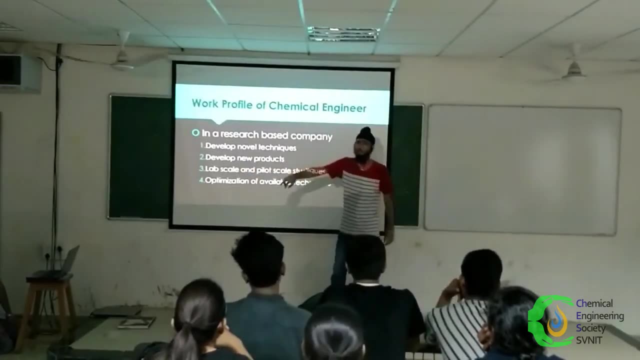 It will be a normal continuous plant, but it will be like smaller in terms of capacity, yield and everything. And then they see that what was applicable in lab scale is giving that much efficiency in pilot scale or not. So that is pilot scale. 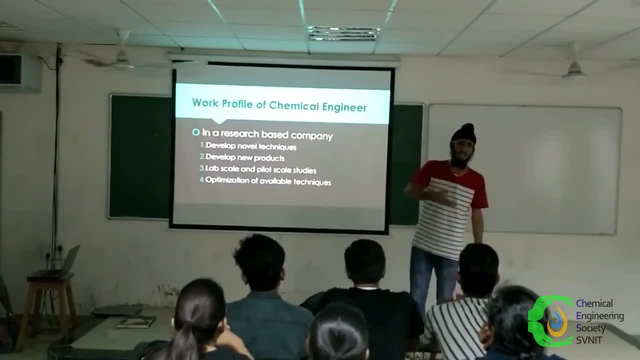 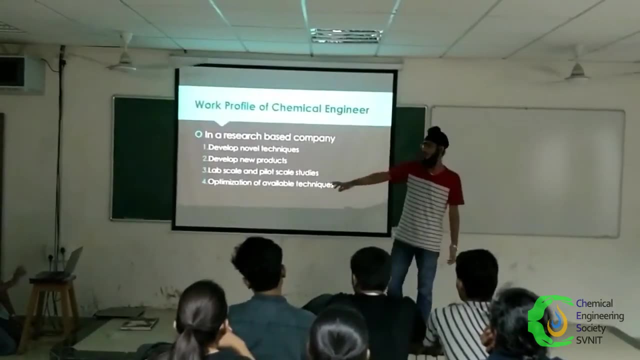 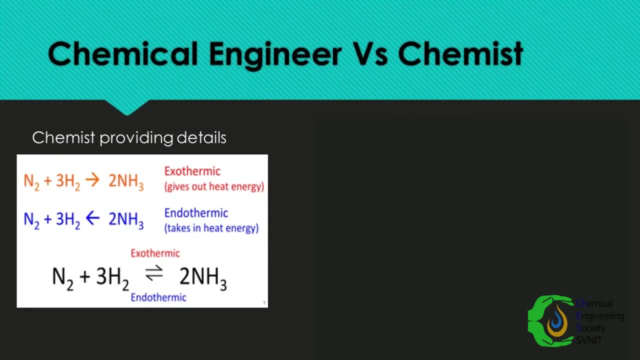 And optimization. optimization means that what I said earlier, troubleshooting, after that, if there is a problem, then they rectify it, rectify it, And that work is also done by design research engineers. Okay, so this is what a chemist.